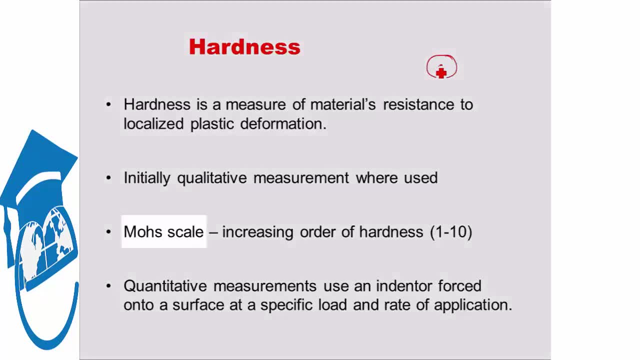 What does that mean? That means that we had something known as Mohs scale. Mohs scale had different materials, beginning from very soft material- Okay, marked at 1, like talc powder, At unit distances 2,, 3 up till 10,. we had different materials. 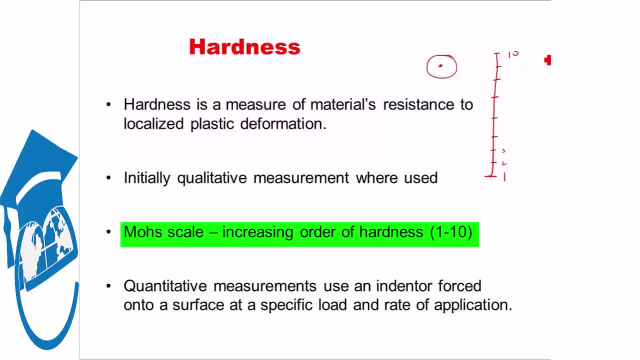 With increasing hardness. Okay, 10 was diamond. Now suppose we took any material, let's say material X, And material X was found such that it scratched the surface of material 4, of material with hardness Mohs scale 4, but it was scratched by that of 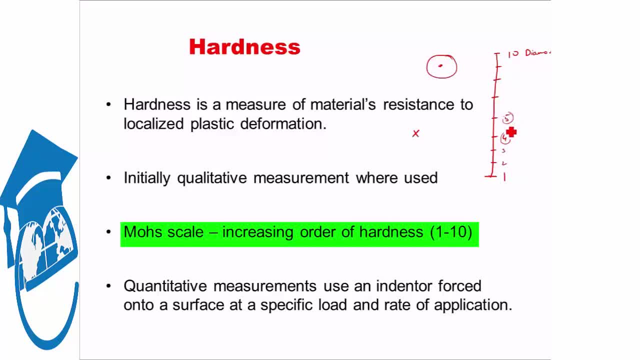 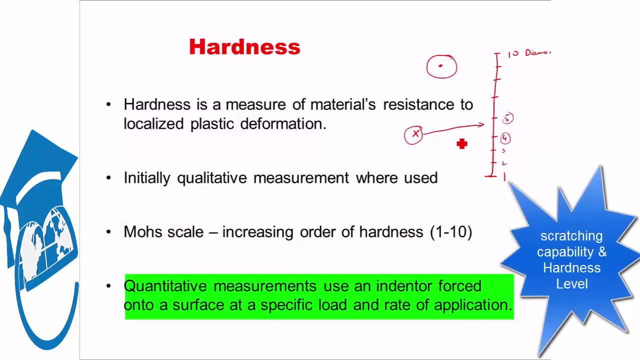 10. Mohs scale 5 hardness. that meant that material X had a hardness in Mohs scale between 4 and 5. so this was a qualitative measurement, right. you compare the scratching capability of two materials and say which one is harder than which material. to begin with you define 10 materials and provide hardness. 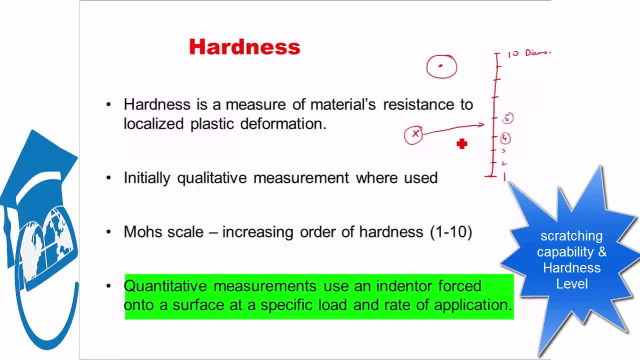 level to each of them and compare a new material with those materials and see where the new material fits. thereby you give a rating. 9 was silicon carbide. so this way there were different materials. this was Mohs scale and this was more of a qualitative approach. okay, there was no specific science, it was more of a 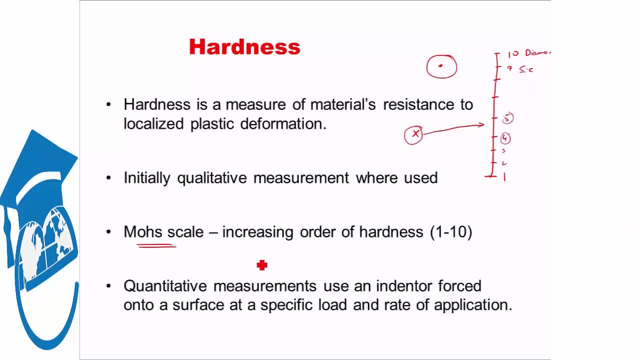 comparison, more of a trial and error kind of thing. but recently- this is the case, not recently. it has been quite a while that quantitative measurements has been done. now, what exactly was the quantitative measurement that was done? that for the quantitative measurement what was done was there were special 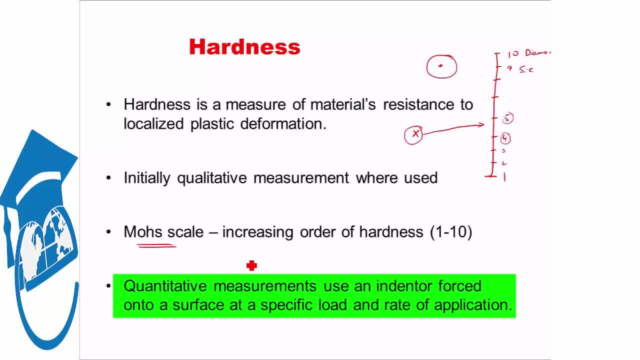 indenters made indenters with specific dimensions which were internationally recognized, and it was decided on specific amount of load and the rate of application of load under those conditions. thus, specially measured material was done. designed indenter was forced into the material whose hardness was to be. 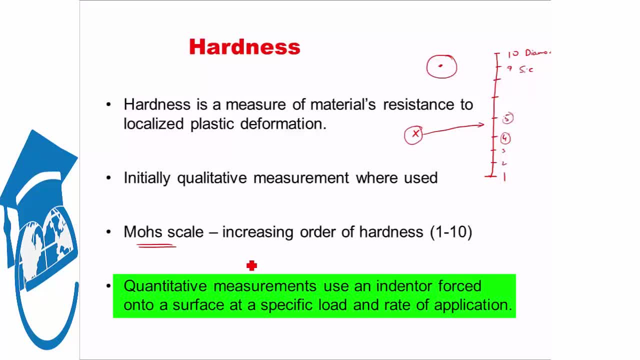 measured okay, and we'll see the different kind of indenters that are available. we'll see the specific loads that are used. so, under this specific conditions of a given indenter, at specific load and specific rate of application, you find out what is the dimension of the indent that is created. 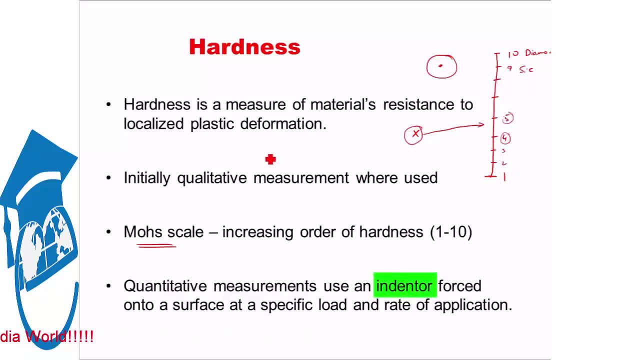 in a material. Now, if the material is soft, then the dimension of the indent that is created will be large, because the indenter will get we penetrated further deep, thereby larger indent will be created. if the material is hard, then smaller indent will be created, thereby medien the dimension of the indent created. we. 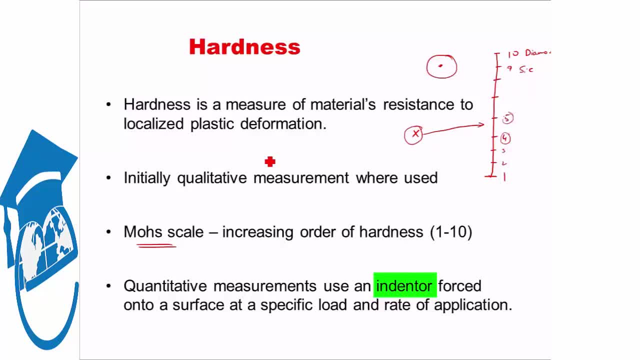 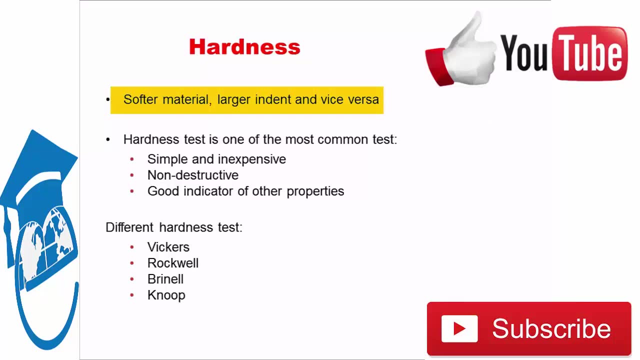 can give it a particular hardness value. that dimension of the indent created is converted into hardness values using specific formulas. that has been derived experimentally. So let us see: Softer material, as I said, will have larger indent, and vice versa. Now what is the importance of hardness test? Why is hardness test so important? What you will see is hardness. 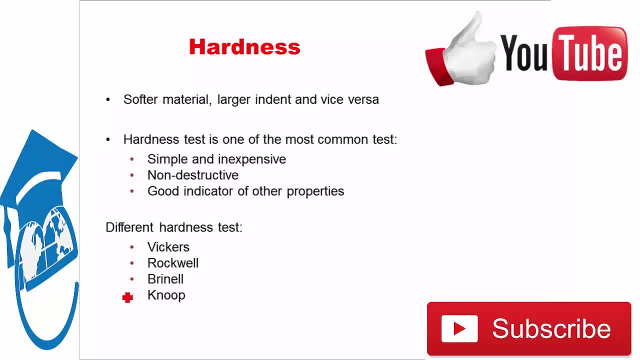 results. hardness of a material is reported in almost all the studies that is carried out. Why so? Because it is very, very simple test and it is quite inexpensive test. But more so, it is a non-destructive test. In the tensile testing, what you saw was you took a specimen, you pulled. 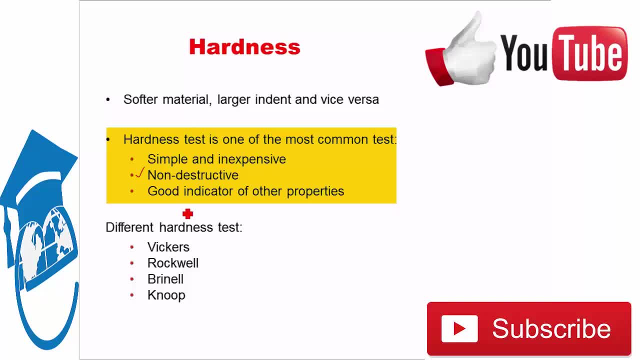 it pulled it till it ultimately failed. So you are actually destroying a material, destroying your sample, But in hardness test you are just creating a very small indent in the specimen and getting a result of a hardness. Therefore it is a non-destructive test and hardness can be related with other properties. 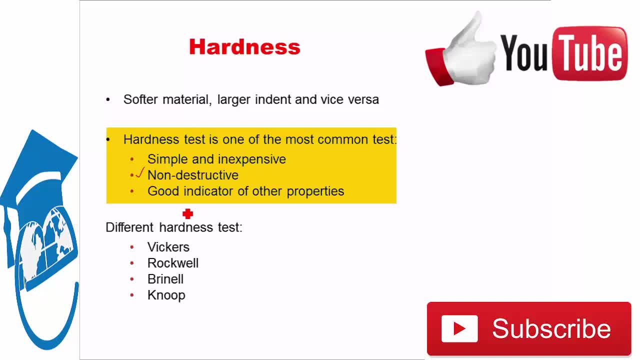 It has found to have good relation with other properties, like tensile properties of the material. Therefore, hardness is a good indicator of the general mechanical properties of a material. So hardness is actually one of the most common test that is carried out for aforementioned reasons. 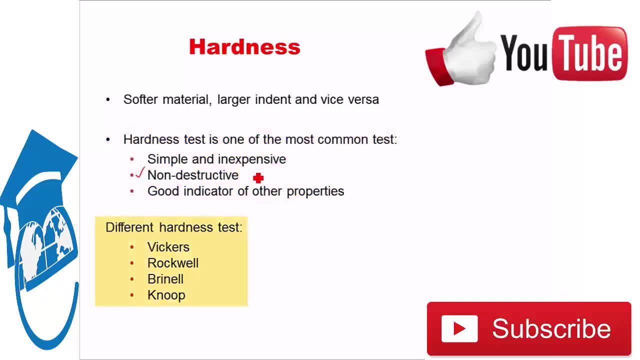 Now, Hardness tests are mainly of four types. Different hardness tests are mainly of four types. One is known as Vickers hardness test. Then we have what is known as Rockwell, Brinell and Knope. We will see each of them in details. 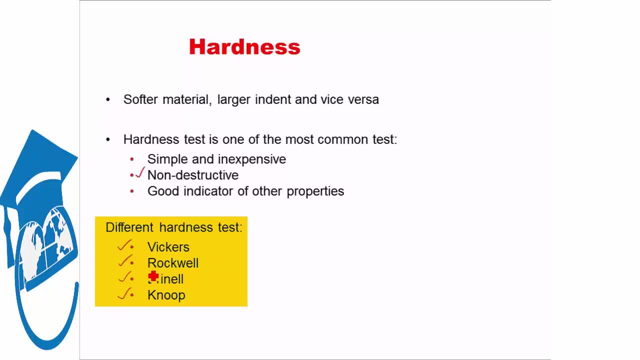 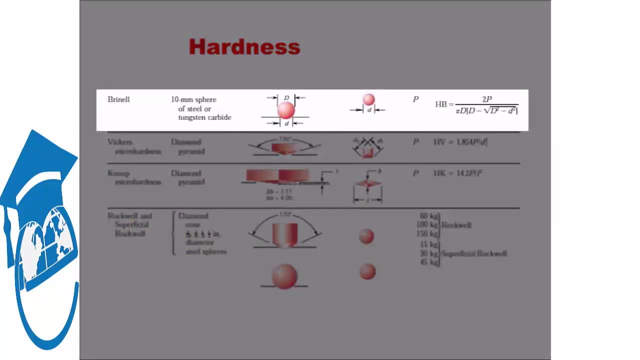 What is the differences between them? under what condition which hardness test is used? Let us see that. Let's start with Brinell. So Brinell is a hardness test in which we use a spherical indenter. The spherical indenter is a 10 mm spear of either steel or tungsten carbide. 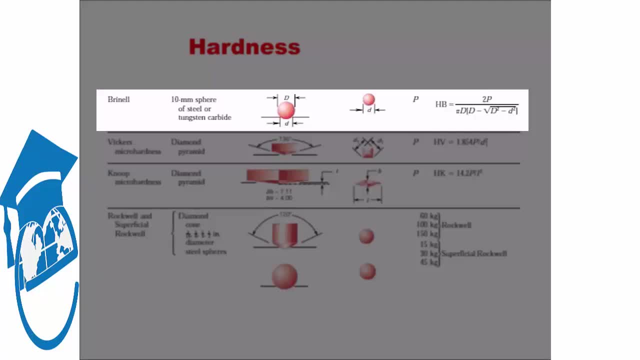 So what this means is we have a spherical indenter which is very, very hard. This is the indenter which is 10 mm across. Now, this is the view. This is the surface of the material. This is the material in which indent is being done. 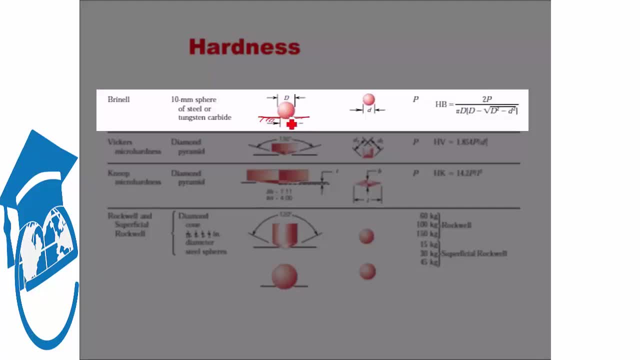 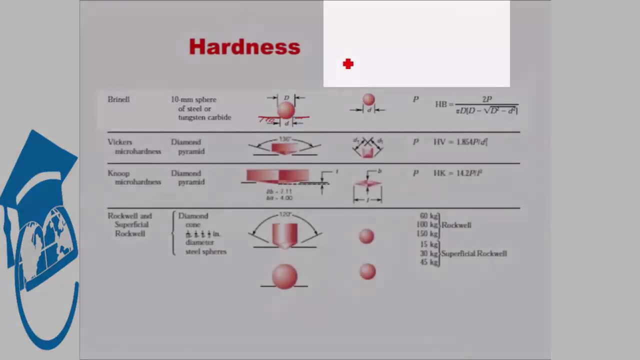 So if the material is very hard, the amount of indent being created will be less. If the material is quite soft, then the amount of indent created will be much larger. So what we can have is either something like this or something like this: 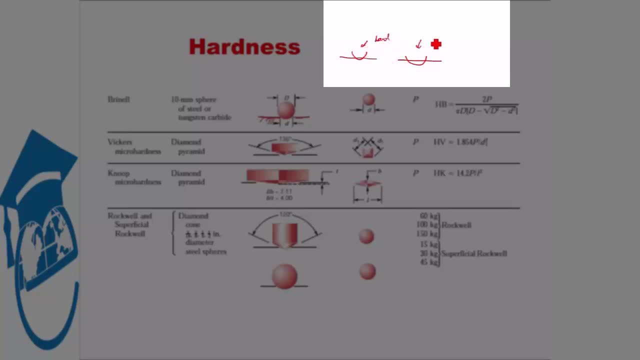 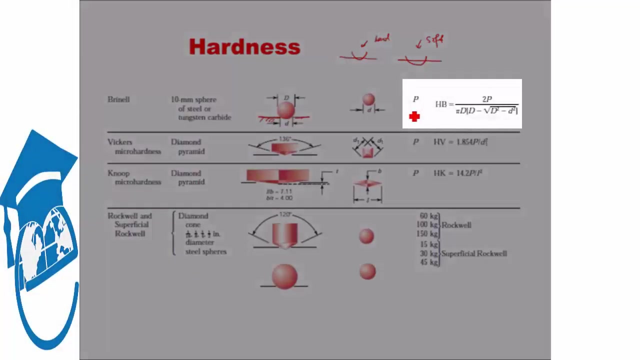 This is hard material. This is soft material, comparatively. So, by measuring this dimension, The radius of the material Indent that is created or the diameter of the indent that is created, We have generated a formula in which we have the value of load. 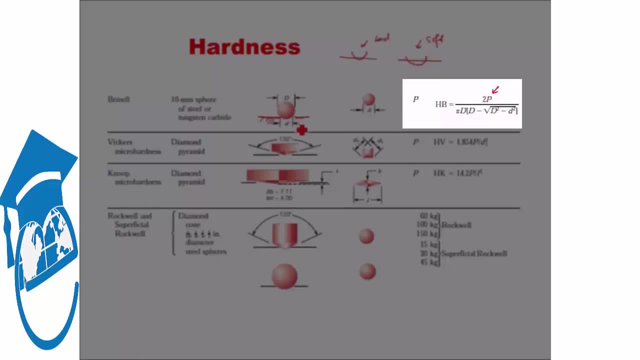 Obviously, more the load you will apply, more will the indent go inside and more will the dimension. So you need to fix the load. or, in order not to worry about the load here, we have already put the load in the formula. Then this is 10 mm basically. 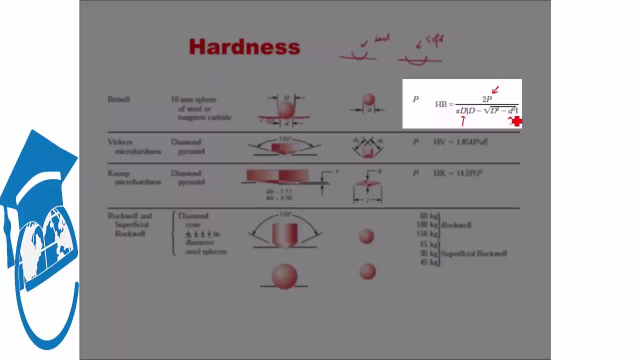 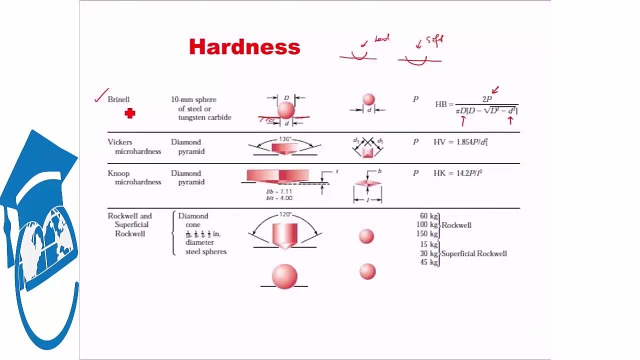 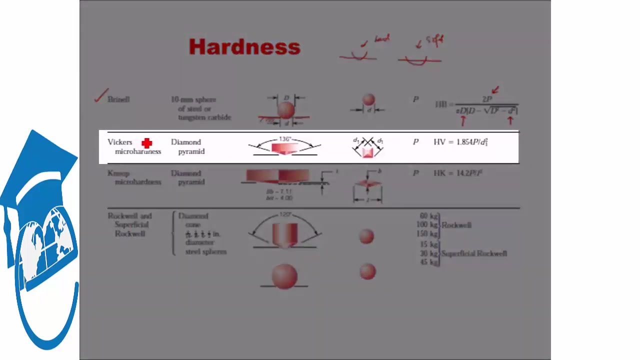 And this is the amount of indent, the dimension of the indent. So more the indent, this whole value will be less. So, as we see, Brinell has spherical indenter. Next let's see what is Vickers hardness. Vickers hardness uses diamond pyramid indenter. 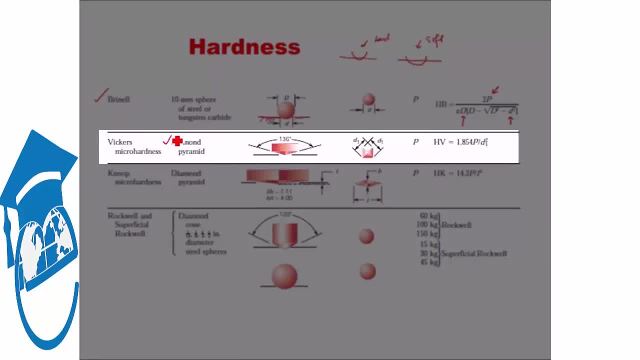 What is diamond pyramid indenter? That means the material Of which the indenter is made is of diamond and the shape of the indenter is pyramid. Exactly how pyramid? The indenter is such that the angle between this surface and this surface is 136 degree. 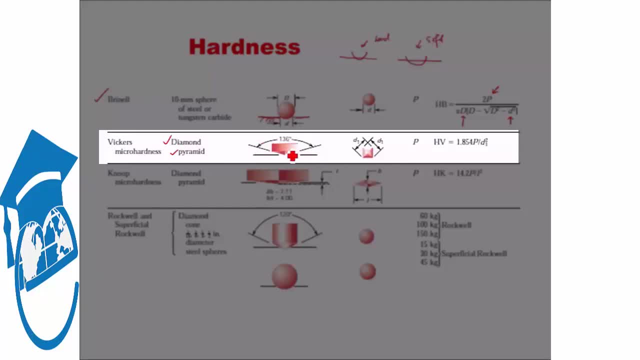 136 degree this dimension and 136 degree between the other two faces too. So the indent that will be created by a Vickers micro hardness tester will be more or less a square in shape. This is going in, so it will create a square in shape. 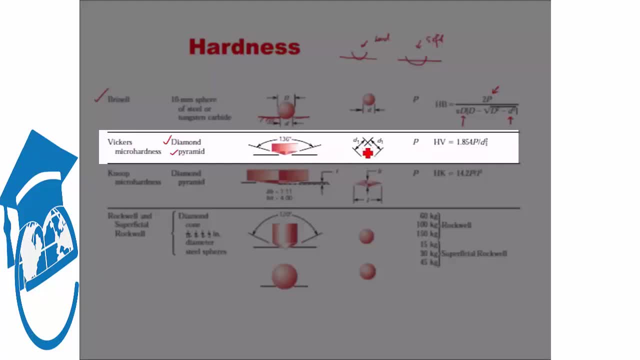 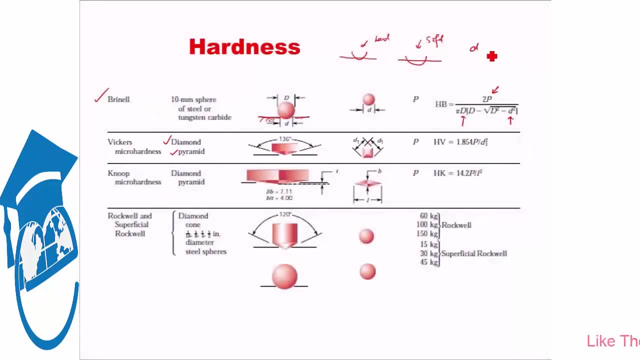 This square- this is the type of indent that we will get- will have two dimension: One diagonal and other diagonal. Let's say, one diagonal is D1 and the other diagonal is D2.. What I will do this two D1 and D2- will be very, very close, but it might not be the same. 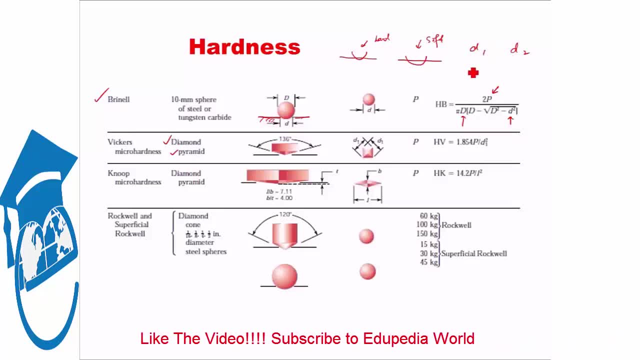 value. So we will just take out the average We will get. D is equal to D1 plus D2 upon 2.. And we plug that inside HV. HV stands for Vicker here, HB stood for Brinell Hardness, Brinell, hardness, Vicker. 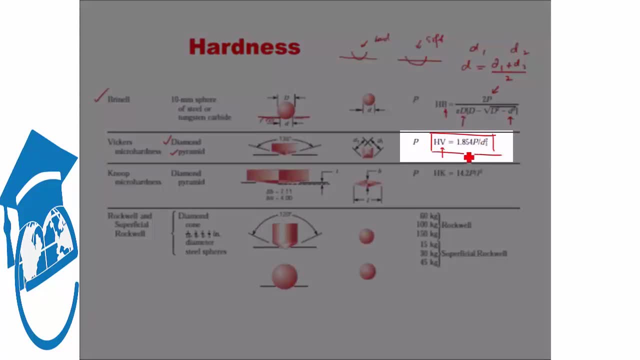 And this is the formula. You need not remember this. These are standard formulas, you can find out by a simple Google. So, but the point to note here is, again, we have the load applied at the top And the dimension of the indent created at the bottom. 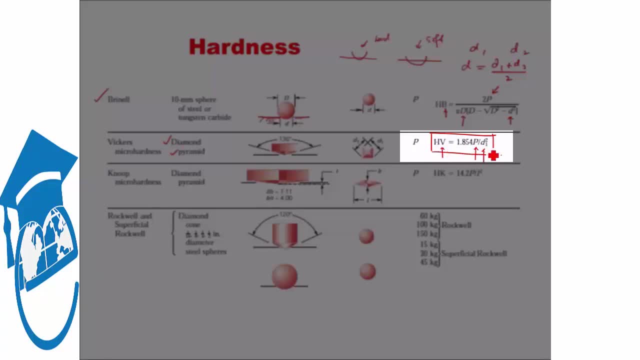 So larger the indent lower will be HV. Smaller the indent higher will be HV. Logically, that is what should happen, Because larger indent means softer material, means HV should be small. Smaller indent means harder material, means HV should be large. 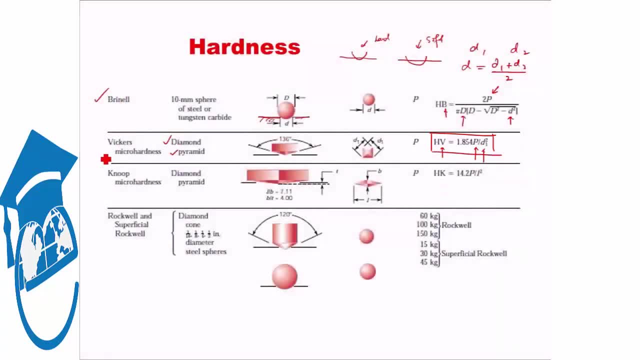 Okay, Now that we have seen Brinell and Vicker hardness, Let's see Noob's micro hardness. Vickers can be hardness or micro hardness, depending on how large the load we are applying. If the specimen is very fragile, we apply a very small load: 1 gram, 2 gram. 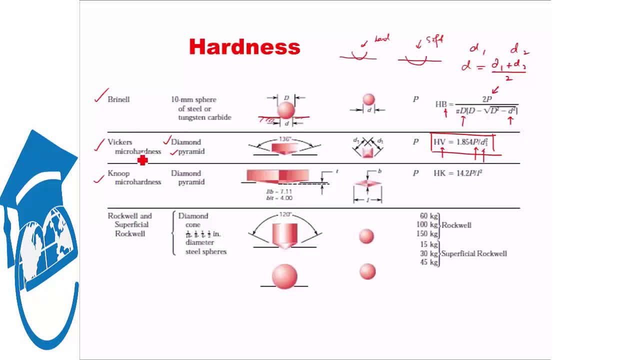 If the material is quite tough, like steel, we can apply 500 grams or 1 kg. So at that time we don't really call it micro hardness, We call it Vickers hardness, whereas Noob's hardness is normally taken For material which are very thin, like: suppose you have a steel in which you have a layer. 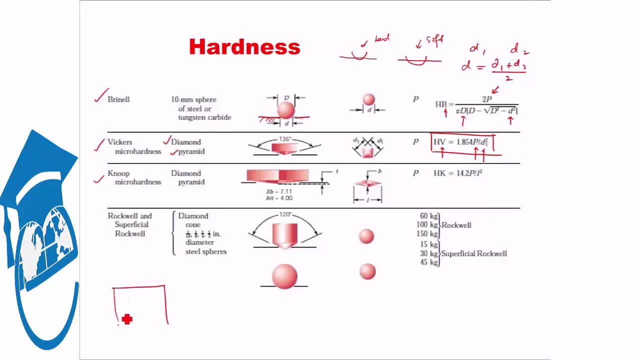 of nitro carburization, or you have carburized it and you want to measure the hardness profile. So what happens in carburization is that basically, carbon diffuses through the surface and the outermost layer will be very hard. as you go in, the hardness keeps on reducing. 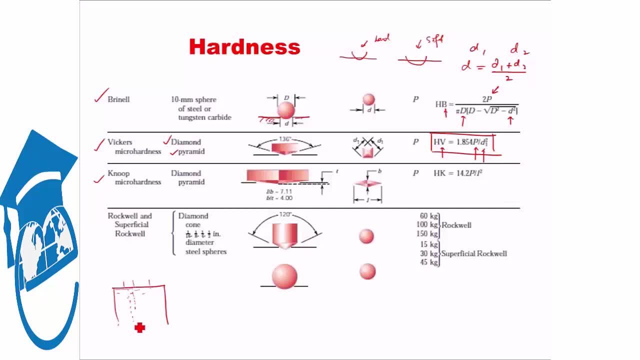 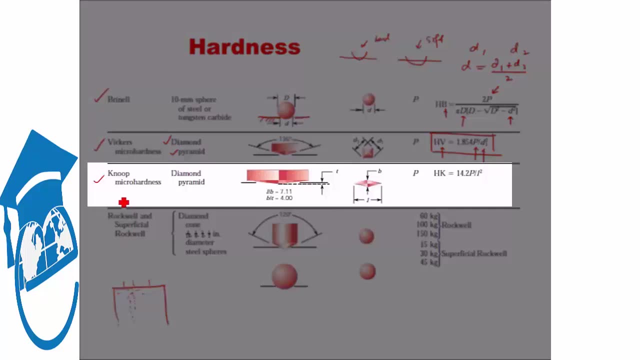 So if you want to profile the hardness With depth, If you use the standard hardness measurement techniques, then you cannot profile it really right because that will create a big indent. You are not really profiling it. But Noob hardness tester, what they have done is that they have created again a diamond. 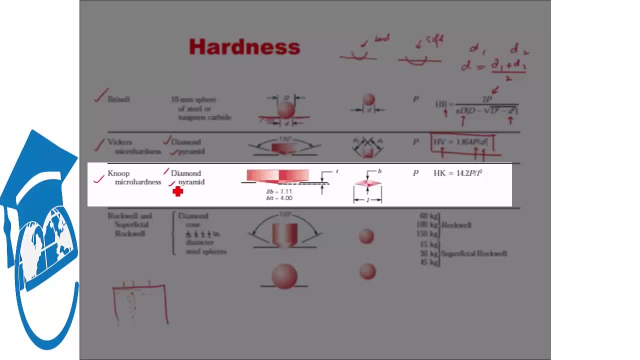 again a pyramid, but the dimension of the pyramid is such that one of the diagonal will be seven millimeters and the width of the other diagonal. Okay, So the length, if it is seven millimeter, the width will be just one millimeter. thereby, 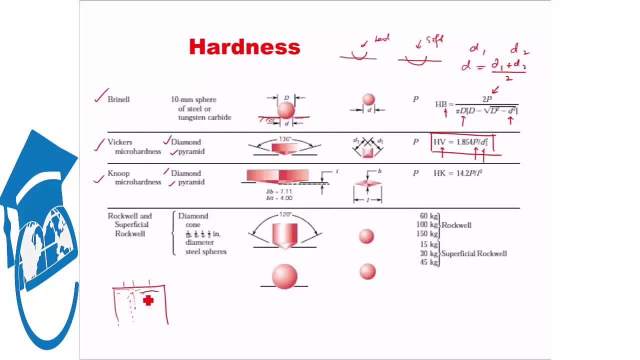 what you can do is that the indent you can take like this. thereby you can get several indents very close by, because this dimension is much lesser. Okay, And that is what Noob hardness tester does. It's mainly used for profiling If there is a different surface or if there is 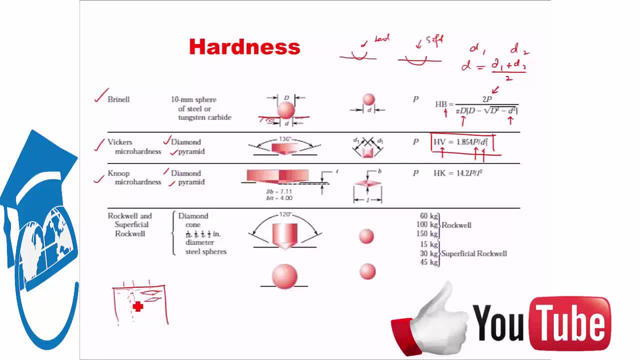 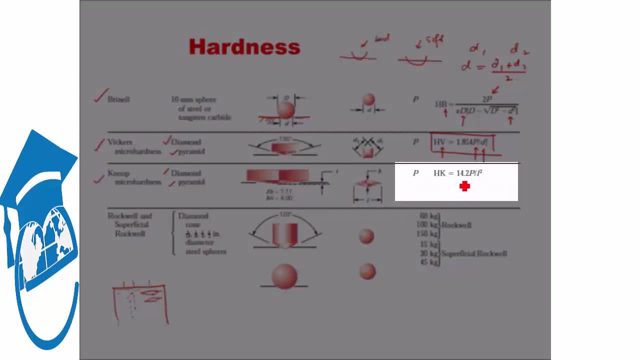 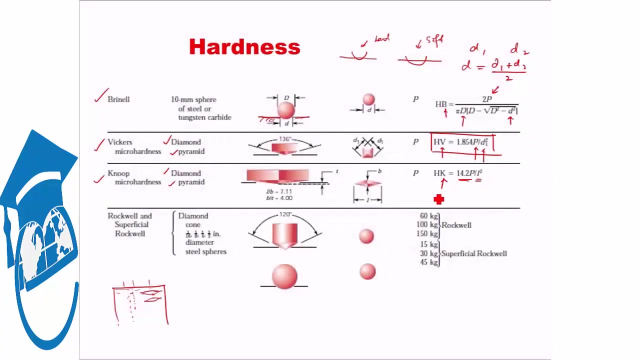 Nitro, carburizing, carbon nitriding, those kind of things. Okay, And again here, what you see is similar to the weaker hardness formula. Here too you have a constant, something load divided by the length square you have taken. So this gives you Noob's hardness, Noob's micro hardness rather. 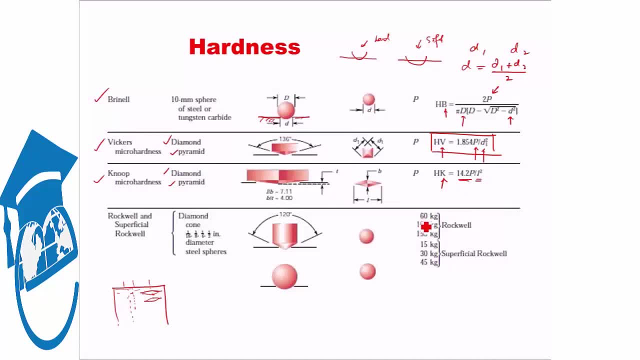 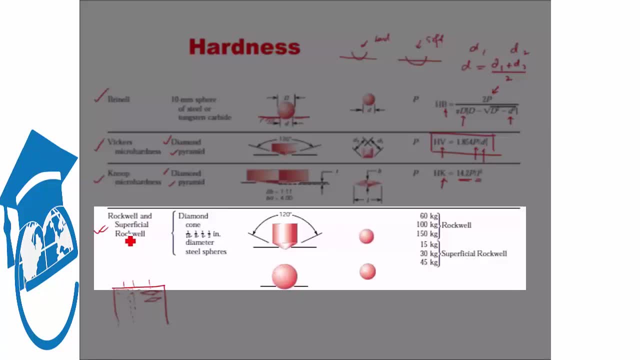 And finally, what we have is one of the Oldest techniques, which is known as the Rockwell hardness test. Rockwell hardness test has a diamond cone. It does not have a pyramid, It does not have a sphere, It has more of a conical shape. 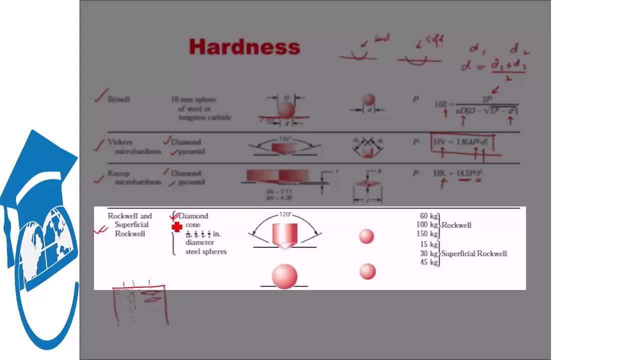 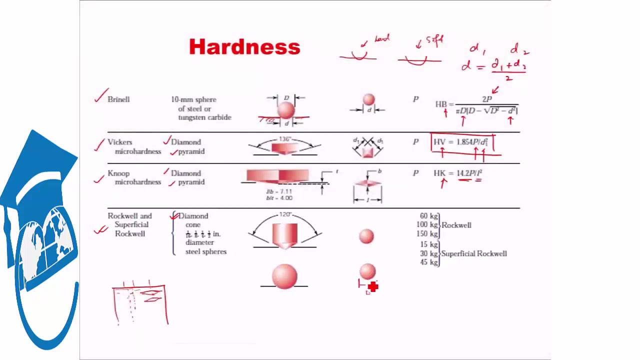 Okay, The conical shape and the diamond material, the cone- will also produce a circular indentation, If you think about it. if you have a cone, it will produce a circular indentation. So here too, You basically measure the diameter of the indent, and we have charts based on which you 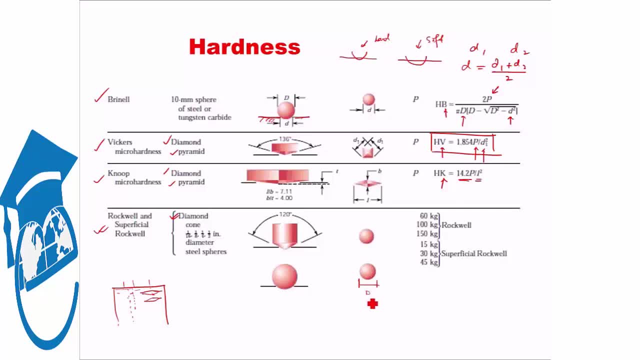 see what dimension corresponds to what hardness. Okay, Now for Rockwell hardness. the thing is that you have some standard dimension of the diamond cone. It's 1, 16th, 1, 8th, 1, 4th, 1, 2nd of an inch in diameter. 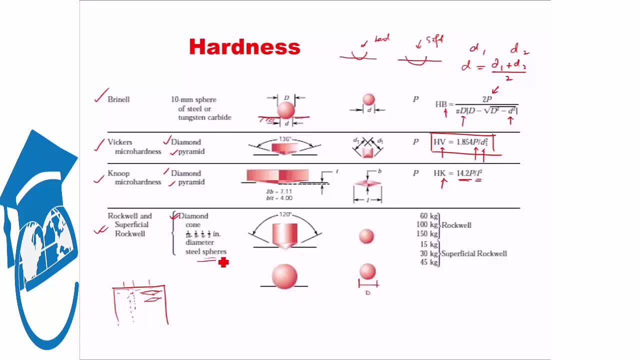 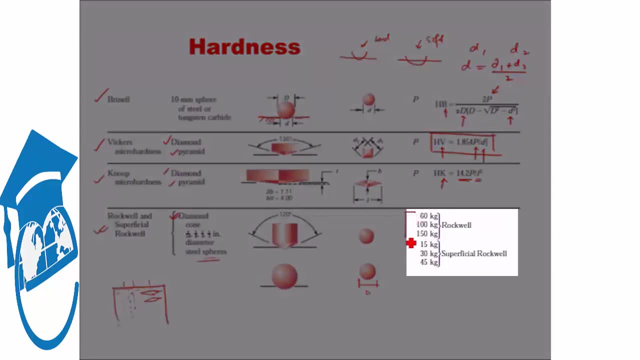 Diamond cone or a steel sphere is also used, Right, So You have a circular indentation Also. you have a spherical indent, rather circular indent, and steel sphere also you have a circular indent. Now the loads that are used in Rockwell hardness are quite high. 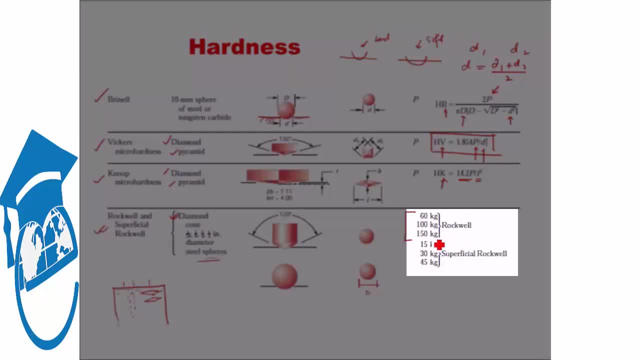 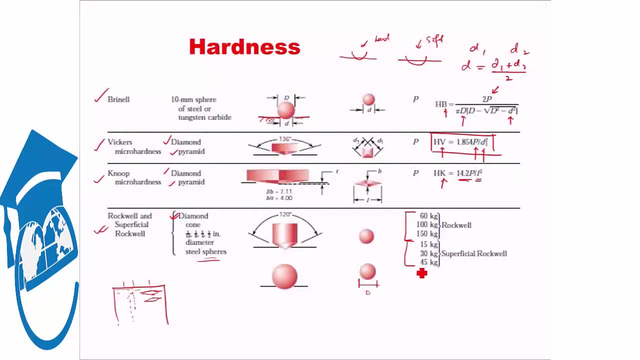 For Rockwell, you have 60, 100 or 150 kg standard. For superficial Rockwell, you have 15, 30 or 45 kg. Using this values, You need to keep in mind that you While Predicting the hardness. 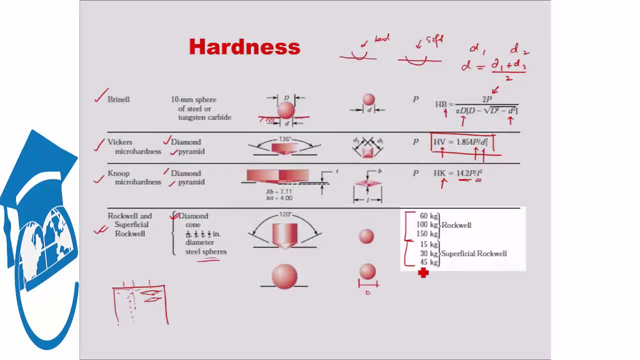 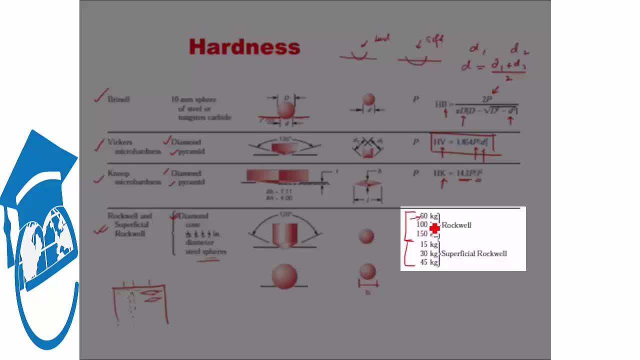 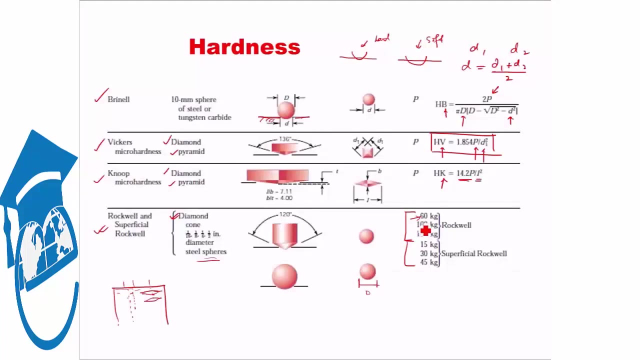 Looking for the hardness from the standard charts, You use the right combination of the dimension and the weight used for hardness measurement. Okay, So these four are the most basic type of hardness measurement: quantitative measurements: Brinell, Vickers, Knope and Rockwell. 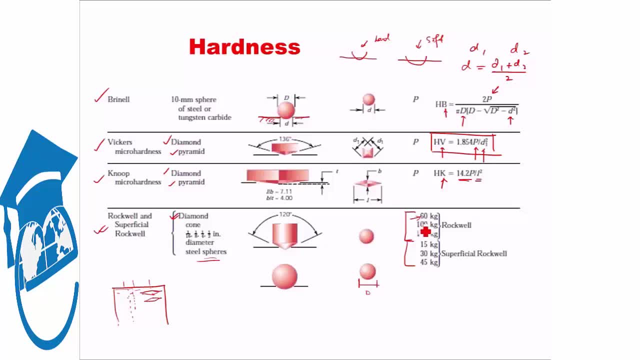 Okay, And there are certain empirical relations between The How to convert one Hardness measurement into other hardness measurement and not going to go into the depth of them. The idea of today's lecture was to give you an idea about what hardness is how to measure. 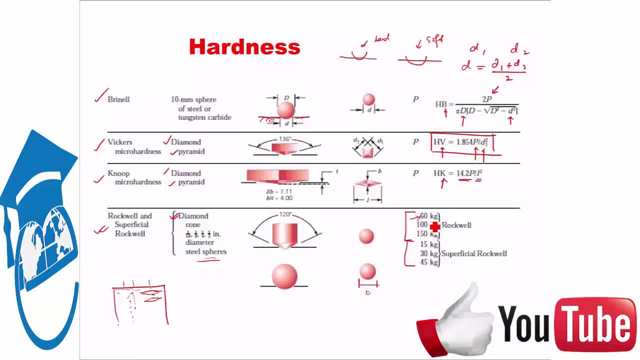 it and what are the standards in the industry that is available for hardness measurement. If you want to study in further details, the the whole idea about the whole next set of lectures And the technical properties is, In fact, in itself a complete coursework.